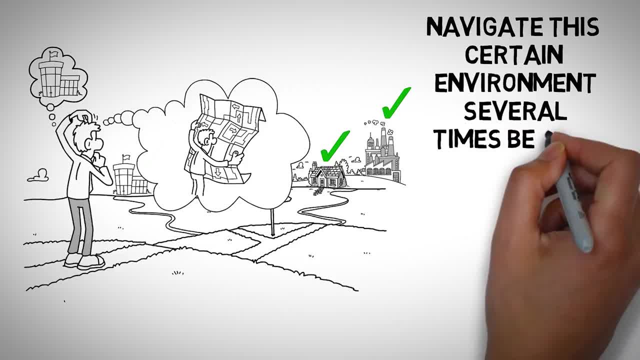 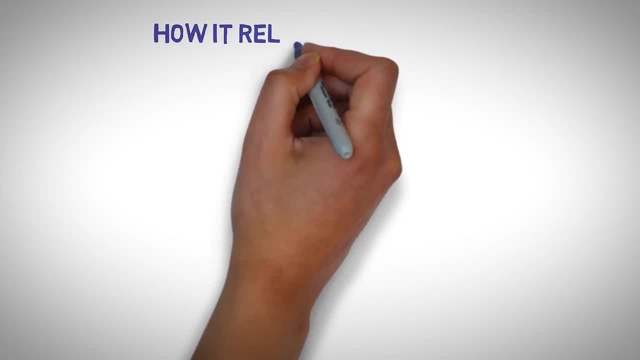 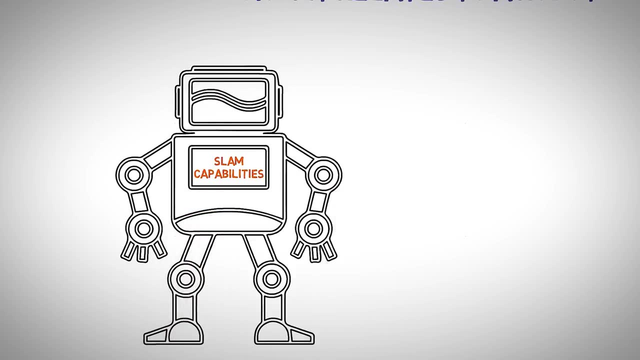 So do you agree that you may have to navigate this certain environment several times before you start becoming familiar with a previously unknown location? So how does it relate to a robot? Now, in the same way, a robot with SLAM capabilities tries to map an unknown environment while 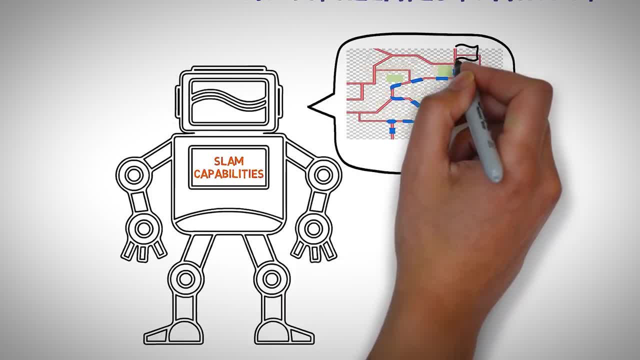 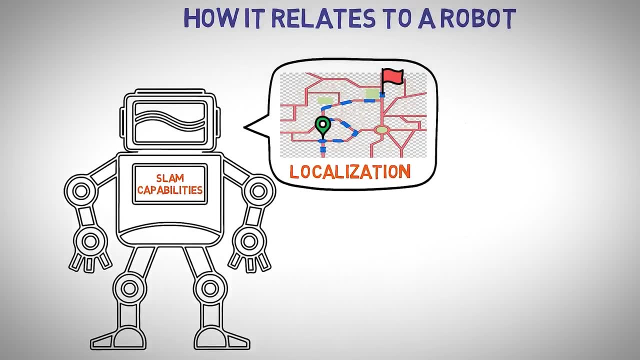 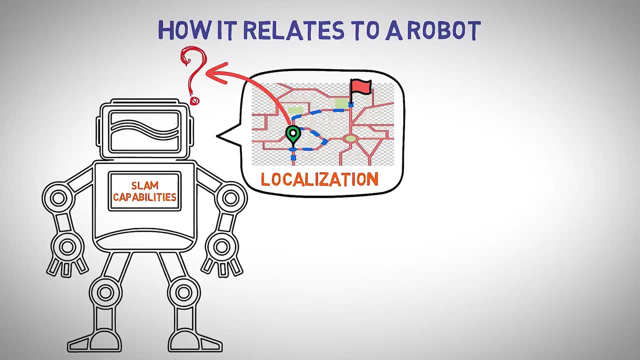 simultaneously trying to figure out where it is at, also known as localization. The challenge comes from doing both at the same time. The robot needs to know its position before answering the question of what the environment looks like. It also has to figure out where it is at, without the benefit of already having a map, Hence simultaneous. 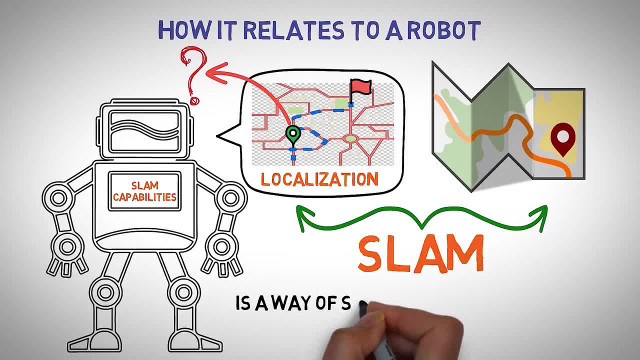 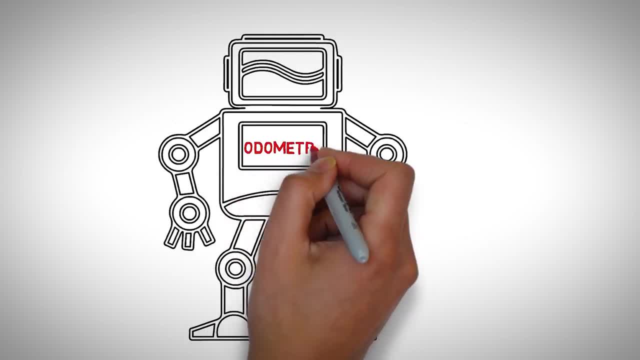 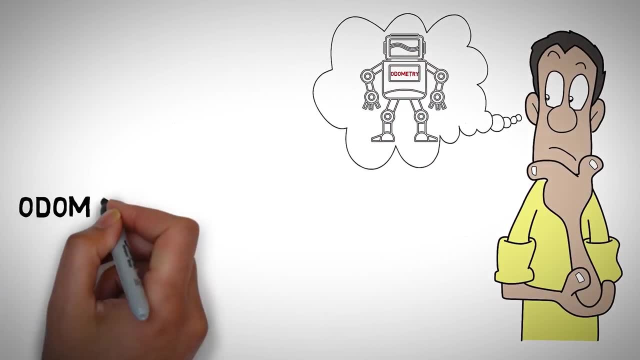 localization and mapping, or SLAM, is a way of solving this problem, using specialised equipment and algorithms. For this process to work, the robot or device must have exceptional odometry performance, So the robot needs to know its location before it can answer. the Odometry is the use of data from motion sensors to estimate change in position over time. 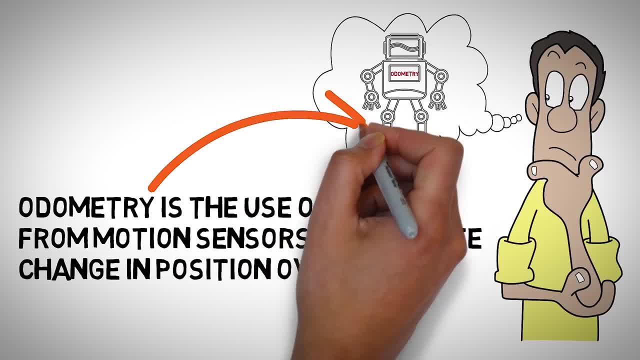 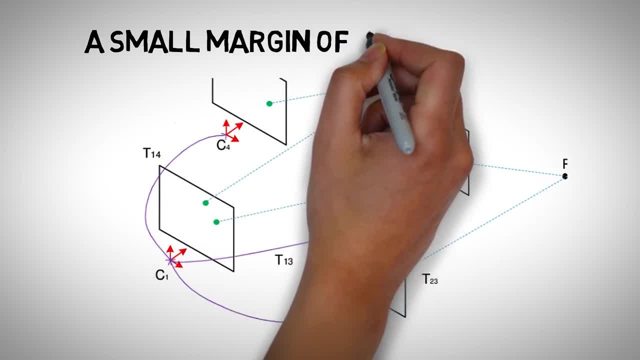 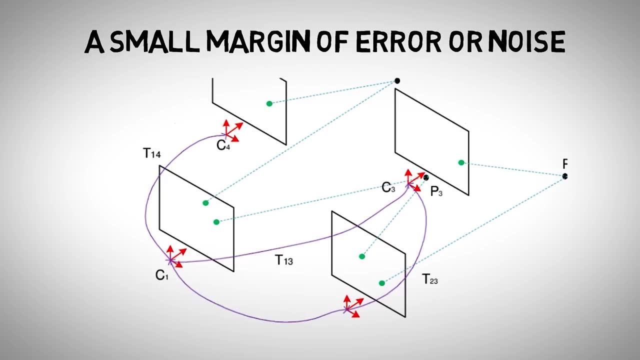 It is used in robotics by some legged and wheeled robots to estimate their position relative to their starting location. With any sort of measurement instrument, there's normally a small margin of error or noise with odometry readings. These errors are taken into account in various algorithms. that also remaps the area to make. 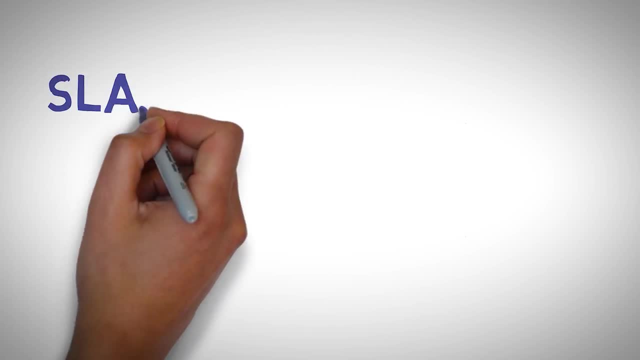 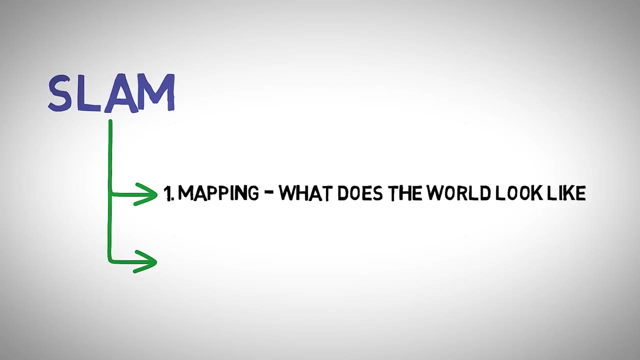 up for this deficiency. So, in a nutshell, SLAM tackles two basic tasks: One: mapping- what does the world look like? Two: localization- where am I? VizSlam, now that we understand what SLAM is now, what the is, VI in VizSlam. 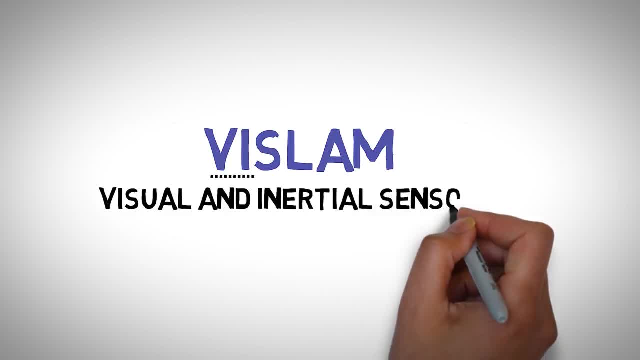 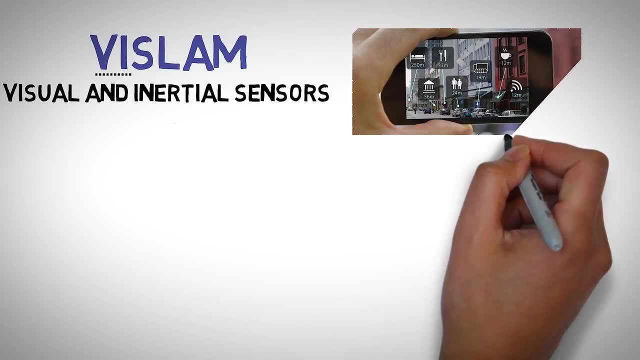 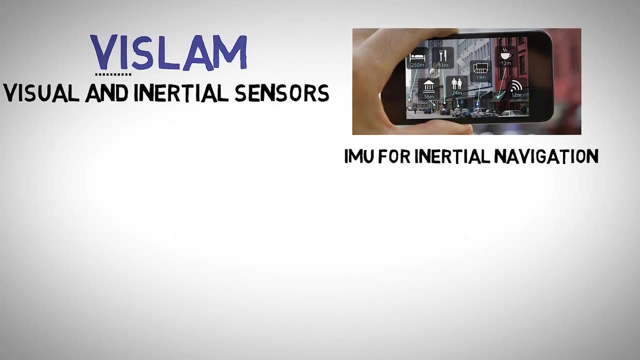 Glad you asked. They are the visual and inertial elements. SLAM can work with a multitude of sensors, But on your smartphone, the only way it can map its surroundings for augmented reality applications is by using the camera and its IMU for inertial navigation. 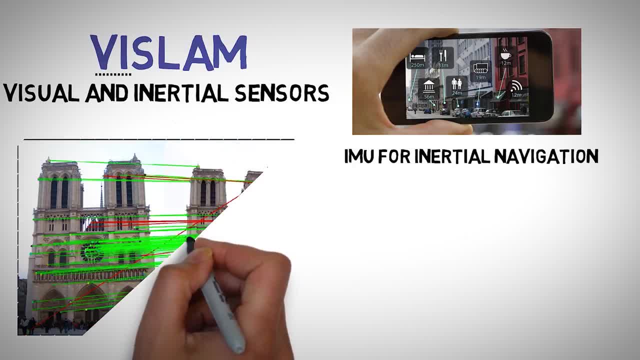 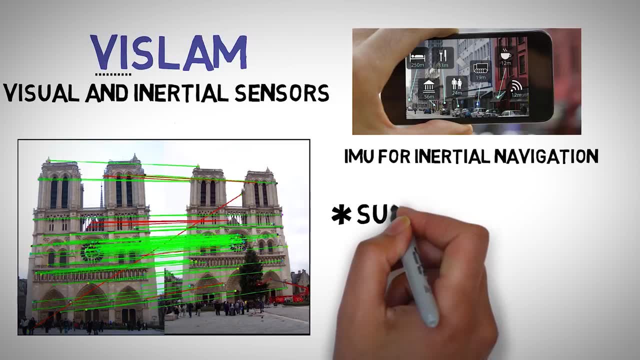 For the visual element. there's a lot of methods that can be used for Bose estimation, But they all essentially try to do feature matching. Some common algorithms that you may or may not be familiar with are SURF, SIFT, Difference of Gaussian AUB, amongst many other techniques. 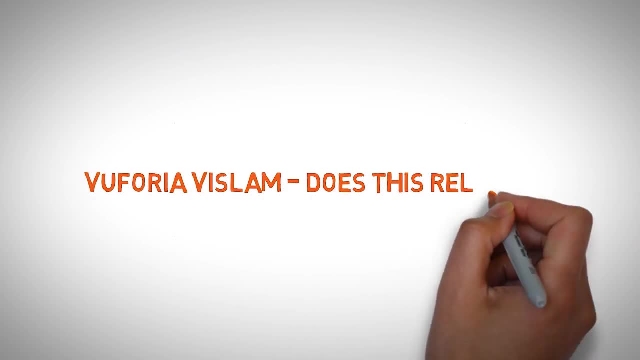 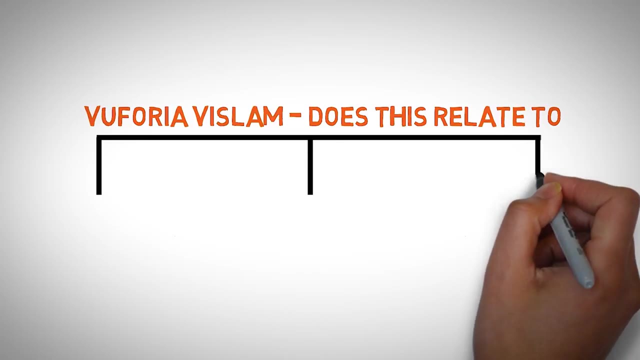 Vuforia, VIzSLAM, and how does it relate to augmented reality? Speaking of augmented reality, Vuforia uses VizSlam in its Vuforia Fusion engine, which enables features such as Device tracker, which provides 6 degrees of freedom in its device. 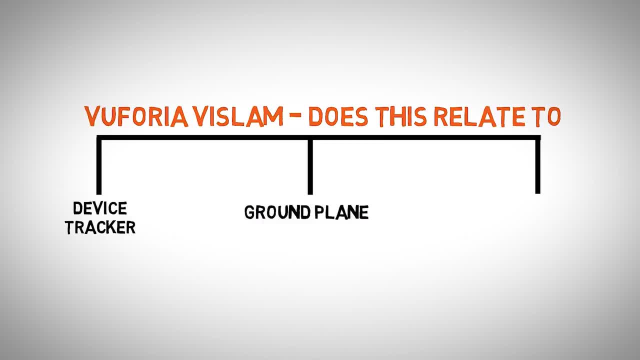 pose Ground plane, allowing virtual content to be placed on horizontal planes in the environment, and extended tracking. Extended tracking is a time- Favorite feature in terms of Hue fra, JUST단��ing and Celsius can essentially run theOnline device into any device. 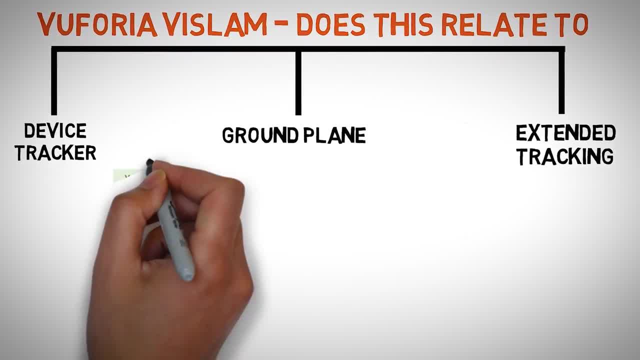 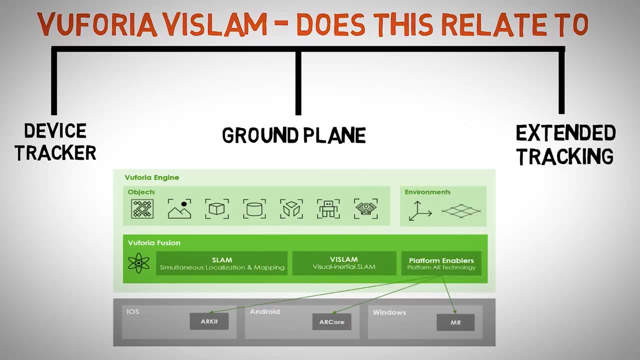 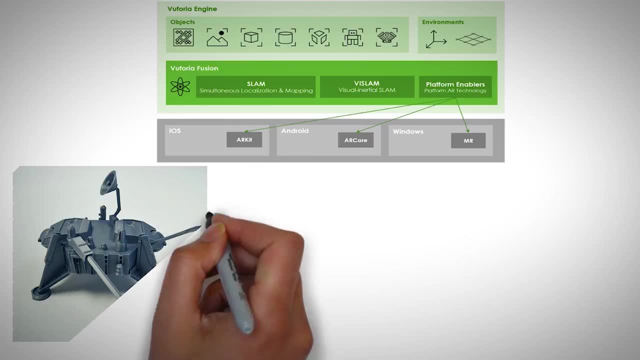 Walls or Terrain. VIFOIA target types. VIFSLAM is an algorithm implemented by VIFOIA combining the benefits of visual inertial odometry and SLAM. VIFOIA VIFSLAM has several benefits: It works better in low-feature environments compared to SLAM-based tracking. 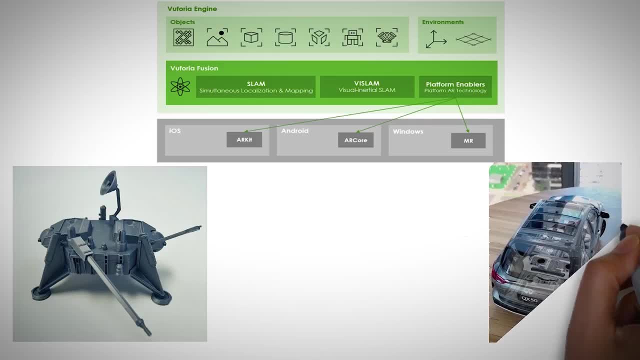 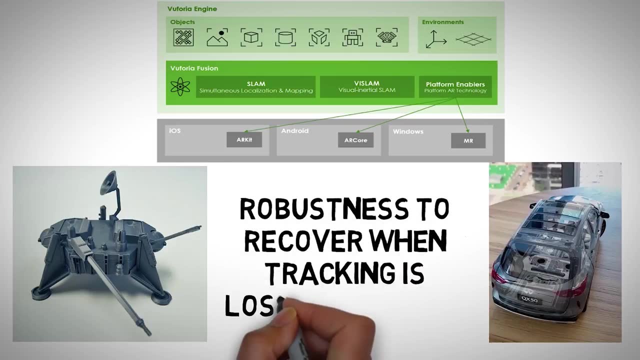 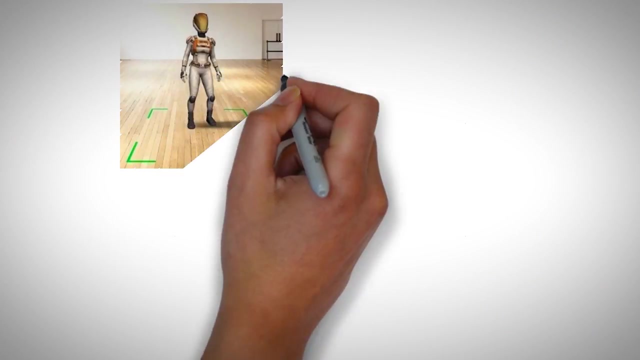 It provides an estimate of the scale of the world, ie the device tracker motion estimate will correspond to the real-world motion And it provides robustness to recover when tracking is completely lost over VO-only solutions. When using ground plane, VIFOIA's VIFSLAM solution will attempt to estimate the distance. 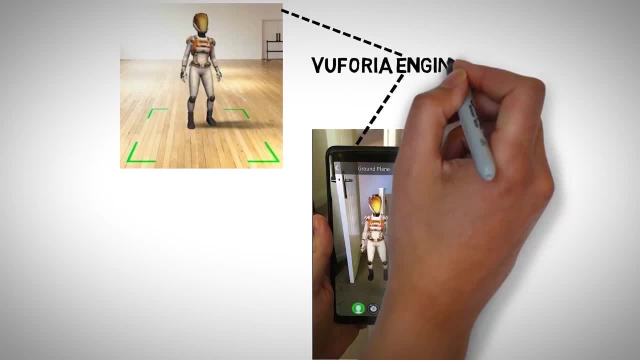 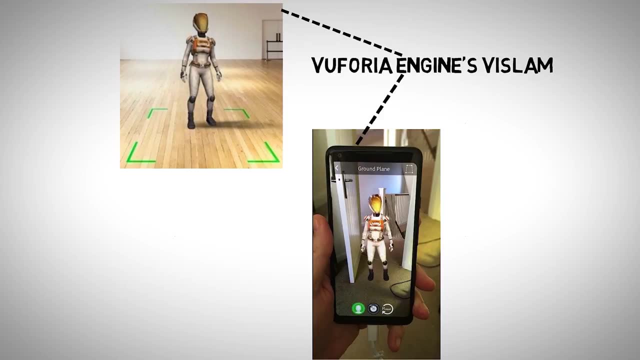 between the camera and the ground plane. To provide a smooth end-user experience, VIFOIA engine will use the initial hints to estimate scale based on the height to the floor provided via the developer API. The default of this hint is 1.4 meters. 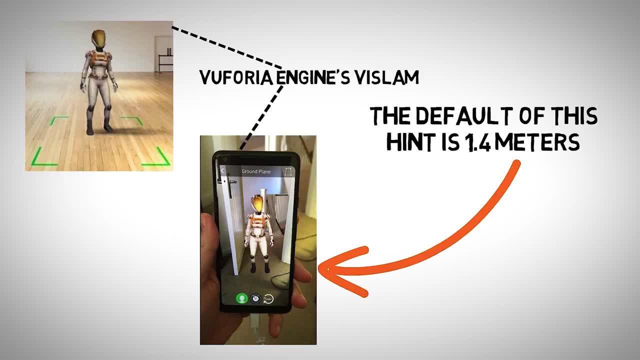 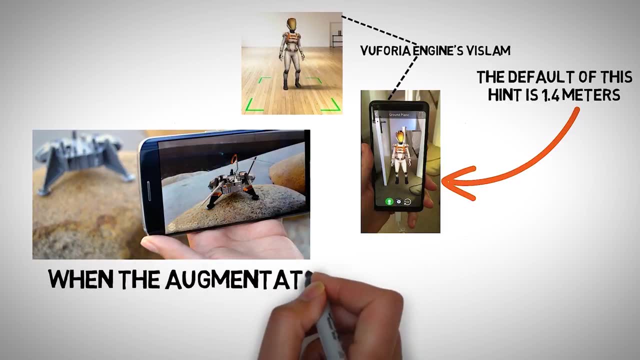 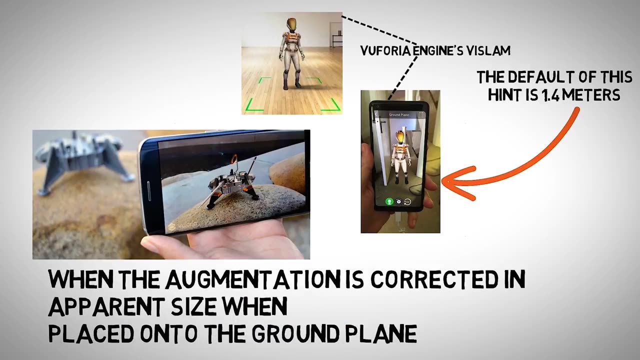 This is the average height of an adult holding a device in their hands. In some cases, you can see the scale estimation at work in the initialization phase of the app, And this is when augmentation is corrected in the apparent size when placed onto the ground plane. 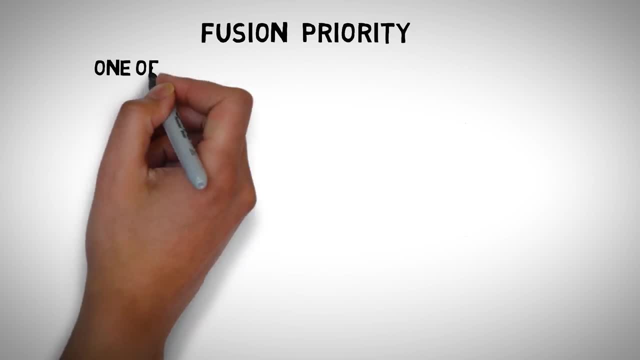 Fusion Priority. So VIFSLAM is just one of the algorithms for AR applications. You are probably familiar with ARKit from Apple and ARKit from Google. It's a very common algorithm for AR applications. It's a very common algorithm for AR applications. 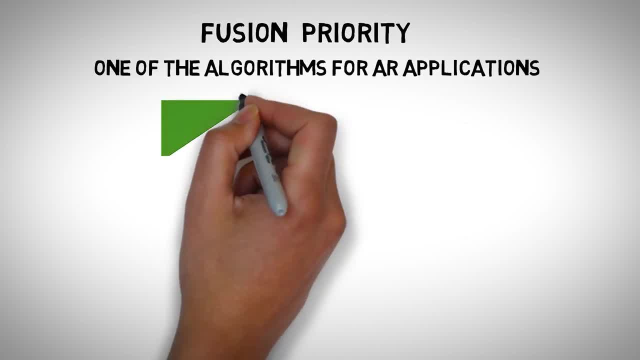 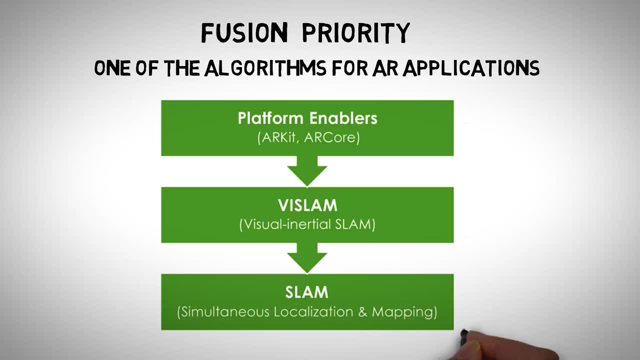 If available, the Fusion API will automatically use ARKit or ARCore. If these platform enablers are not available on the user's devices, it will automatically use VIFSLAM if the device has the required sensors and has been calibrated by VIFOIA.